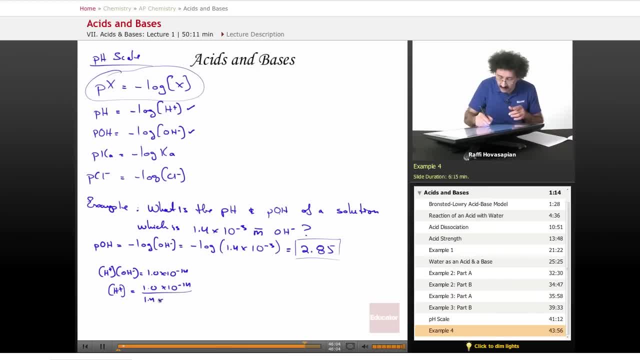 14, divided by 1.4 times 10 to the negative 3. That's going to equal 7.2 times 10 to the negative 12.. And then when I take the pH of that, that's going to be the negative log of the H concentration. 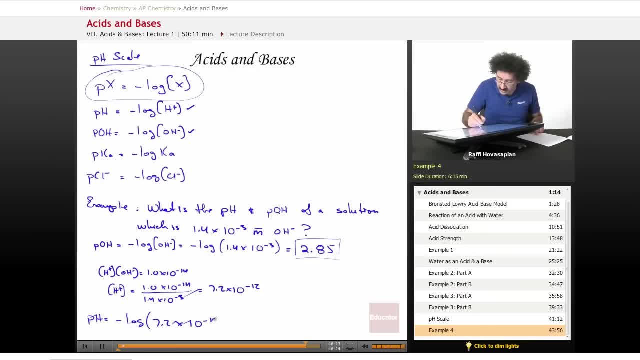 negative log of 7.2 times 10 to the negative 12 equals 11.14.. pH, 2.85, pOH- Notice something? What is 11.14 plus 2.85?? Yeah, you guessed it, It's about 14.. 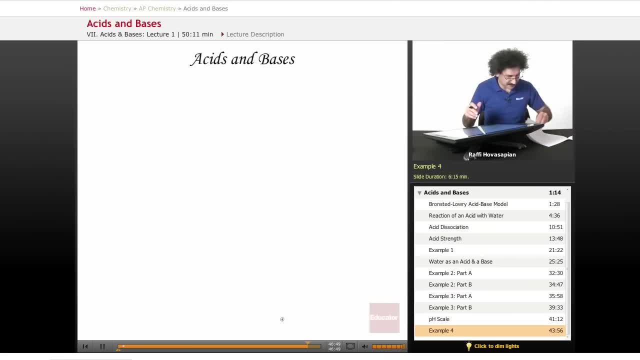 Now let's explain why We said that Kw is equal to the hydrogen ion concentration times the hydroxide ion concentration. Let's take the negative log of both sides. Negative log of Kw is equal to negative log of this whole thing: H plus OH minus. Well, negative log of Kw is pKw, That's it. 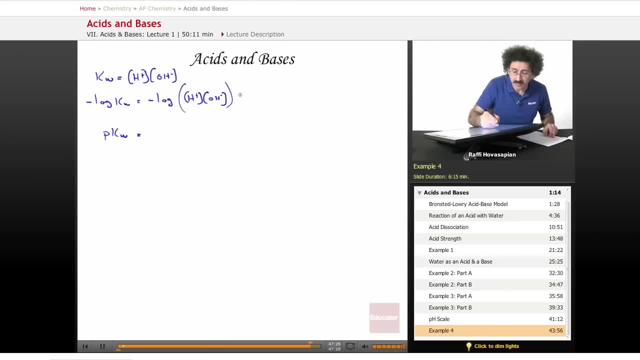 Equals negative log of H, that's equal to negative log of H plus right, Plus the negative log of OH minus. You end up with pH plus pOH. Well, pKw is the negative log of 1.0 times 10 to the negative 14. 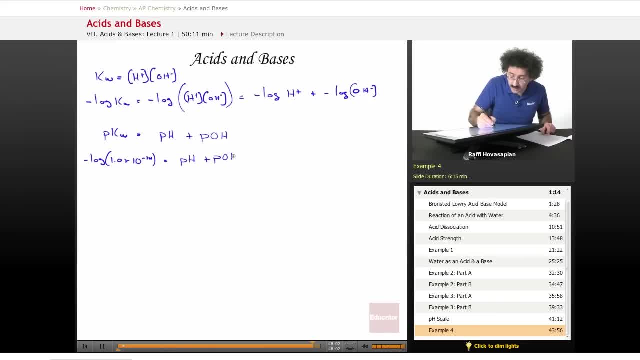 poH equals pKw, pH plus pOH, because Kw is 1 times 10 to the negative 14.. The negative log of that is 14.. That's our final relationship. So for any aqueous solution at 25 degrees Celsius,